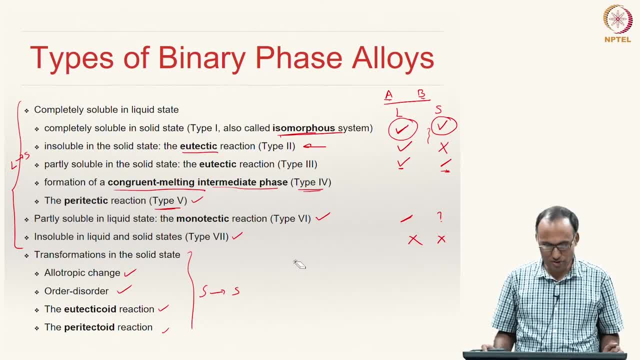 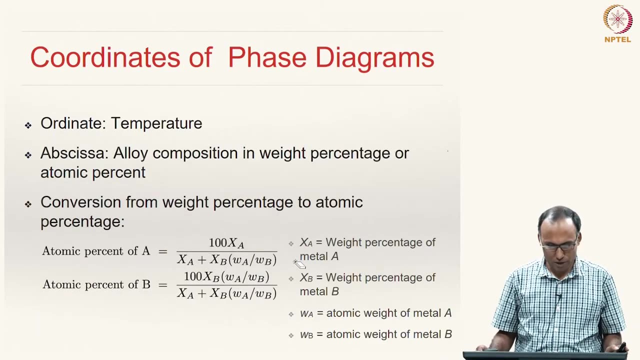 discuss in this class, followed by some solid state phase transformations. Then we will finally spend some time understanding important phase diagram for us called iron-carbon equilibrium diagram. So before we actually start looking at phase diagrams themselves, we need to see how these phase diagrams are drawn. So phase diagram: 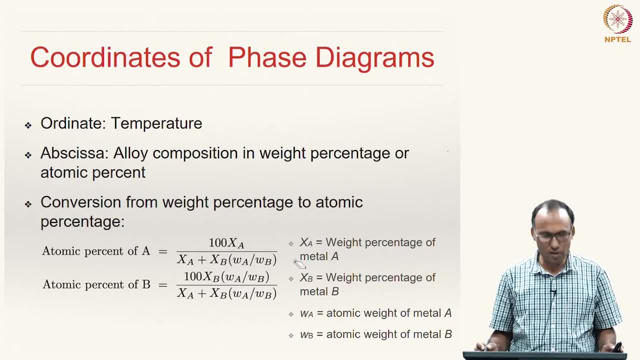 is a…. Here we have two variables like temperature and composition. So on the y-axis ordinate, you will have temperature and in x-axis you will have the alloy composition. The alloy composition can be written in weight, percentage or atom. 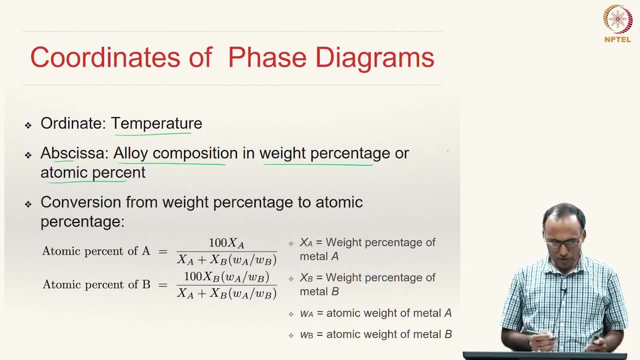 percentage right, And we know how to convert from weight percentage to atom percentage. Usually, when we look at phase diagrams, the typical phase diagram looks something like this: So on the y-axis you have temperature and on the x-axis you have weight percentage. 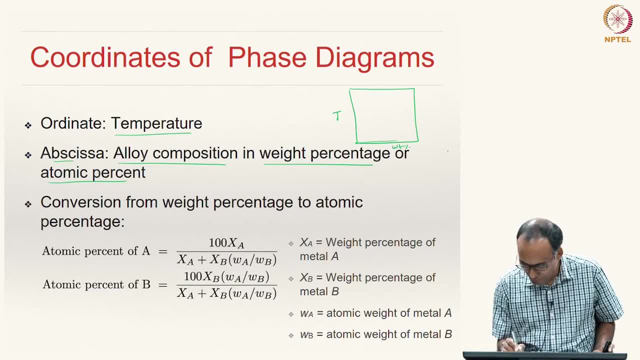 How is it drawn? So the weight percentage? suppose, if you have a weight percentage of, say, element b, So that means, here element b is 0. That means, element a is 100. And here element b is 100. That means, element a is 0. So usually only one variable is shown: element b or element. 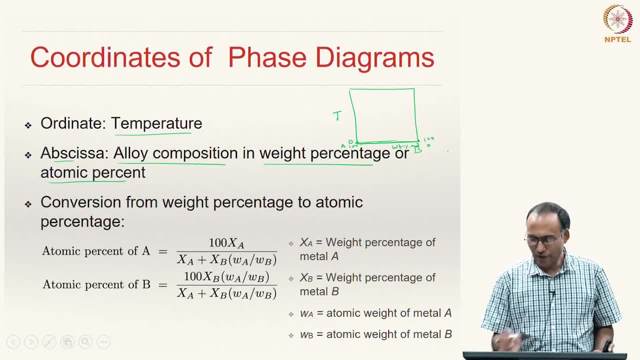 a and then we are going from 0 to 100 weight percent. Similarly the many times on the same phase diagram you will use the top x-axis for atom percentage. So the phase diagram, same phase diagram can be used, can be read both in weight. 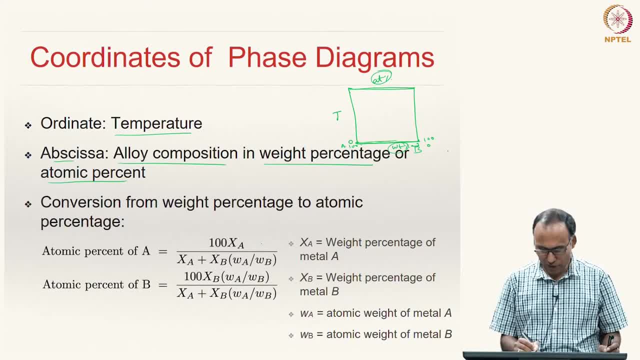 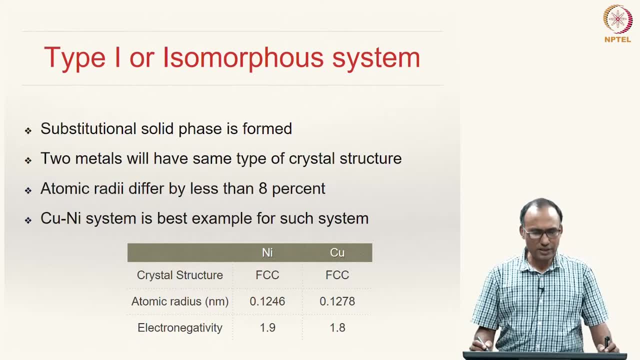 percentage as well as atom percentage, And always we know the conversion from weight percent to atom percent and vice versa. So now we look at type 1, or isomorphous alloys. So isomorphous alloys are the ones which have complete solubility in solid state as well as liquid state. As we look at type I, 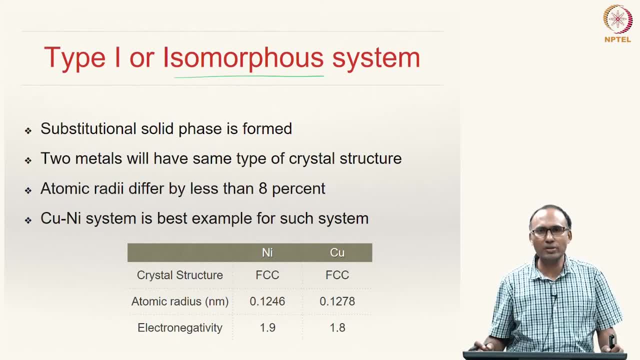 we have looked at the Hume Rothrich's rules. 100 percent solubility is possible only when the atoms are of similar sizes. When the atoms are of similar sizes, then it is more probable to form a substitutional solid solution, because forming an interstitial solid solution will 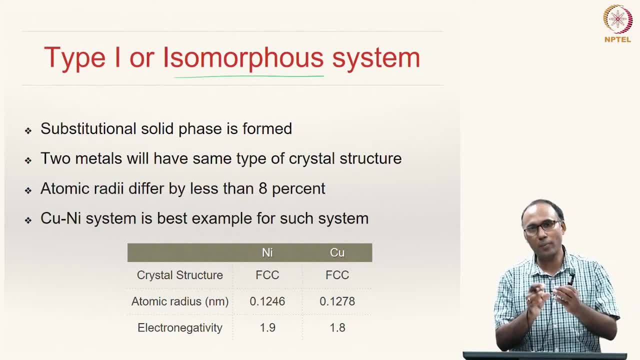 be very difficult because you need to create lot of distortion amongst the interstitial locations, because the atom size itself is larger And hence usually all our isomorphous systems are substitutional solid solutions. We will have a substitutional solid phase And because it has 100 percent solubility according to Hume Rothrich's principles rules. 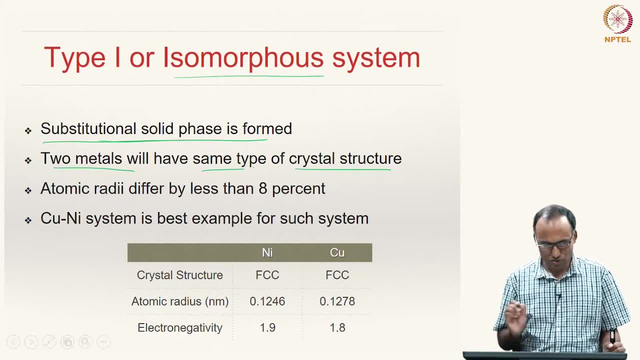 you should have both the metals with the same crystal structure, So the two metals will have same type of crystal structure and atomic radii difference should be less than 8 percent. So, with all these characteristics, a very good example of isomorphous system is the: 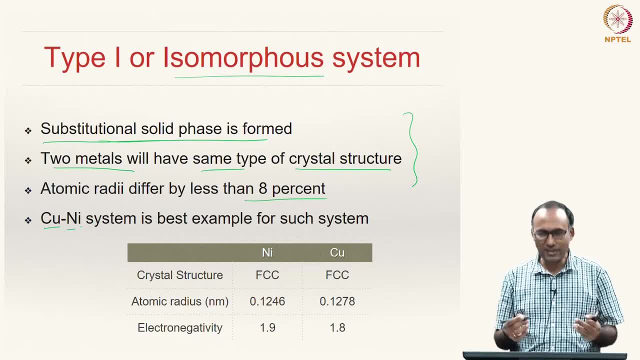 copper- nickel system. So copper and nickel. why they form an isomorphous alloy system? Because you can see the nickel and copper both have FCC crystal structure. The atomic radius are very close: 0.1 to 4- 6 and 0.1 to 7- 8, less than 8 percent difference And their 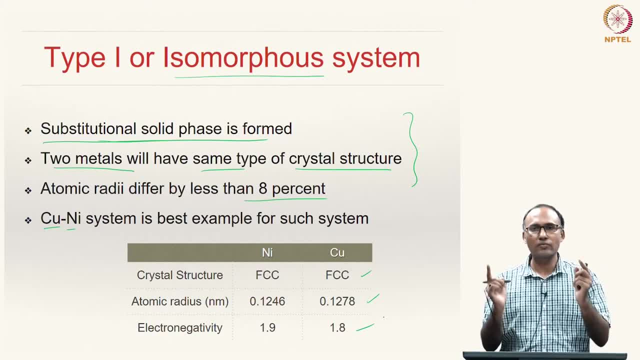 electronegativity values are also very close. That is also another requirement for having 100 percent solubility. The electronegativity is also should be very close to each other, And hence copper nickel system forms a very good substitutional solid solution. So this: 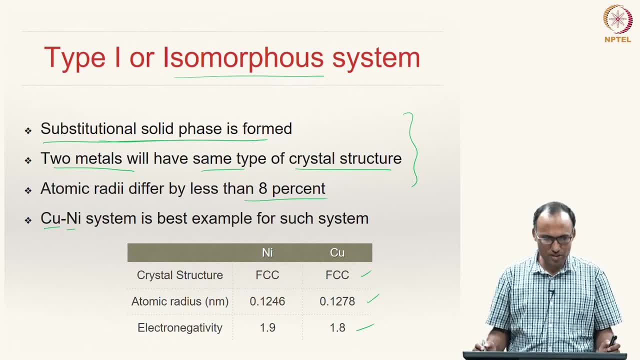 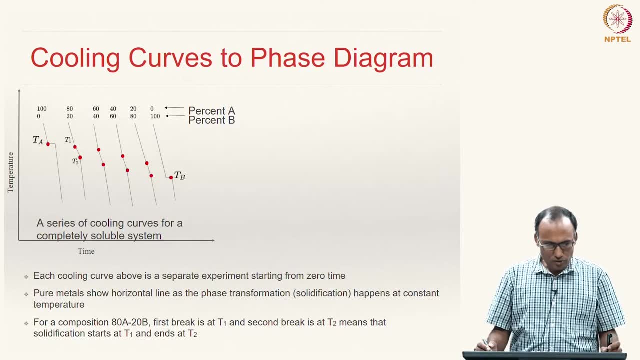 is also a very good example of an isomorphous system. Thank you very much. Thank you very much. good example system or model system for understanding isomorphous alloys. So here in this course we will start trying to understand phase diagrams from cooling. 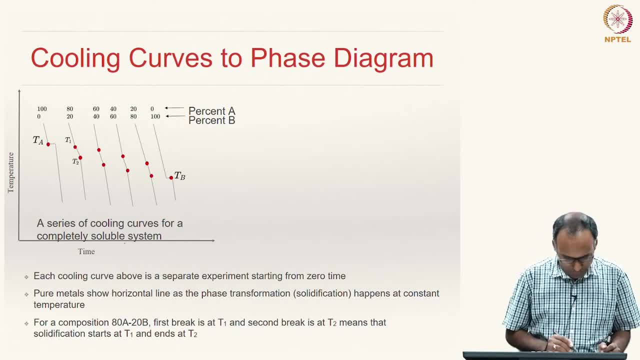 curves right away. So here on the left hand side, you have temperature as a function of time, temperature versus time. And now here each of these lines represent cooling, represent the transformation. or suppose, if you take this pure metal, A, that is 100 A. So here, 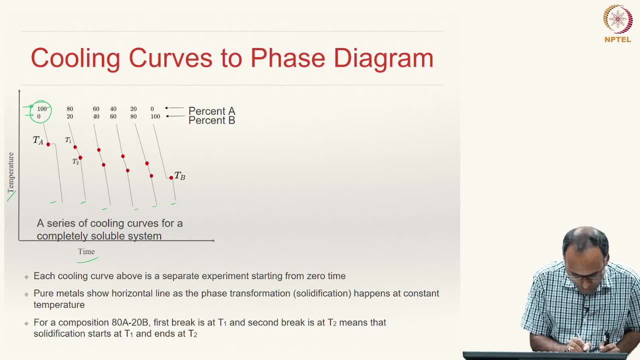 this top line represents percentage of A, weight fraction of A and bottom line represents weight fraction of B. So when it is 100 and 0, that means it is pure metal A. and then the pure metal A is from a very high temperature, which is in liquid state. 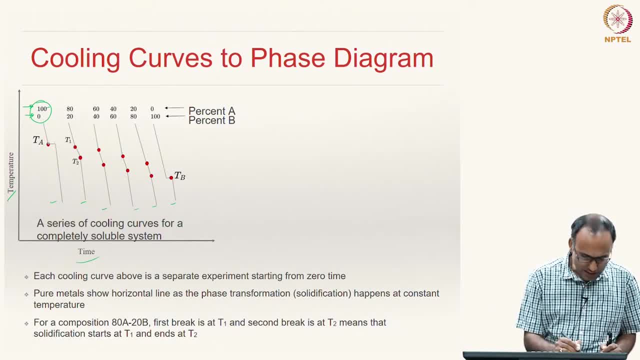 It is cooled down The moment it reaches the solidification temperature of A, T, A. let us say metal A has higher melting point than metal B. So as soon as it reaches its solidification temperature at constant temperature it solidifies, It gives latent heat of solidification. 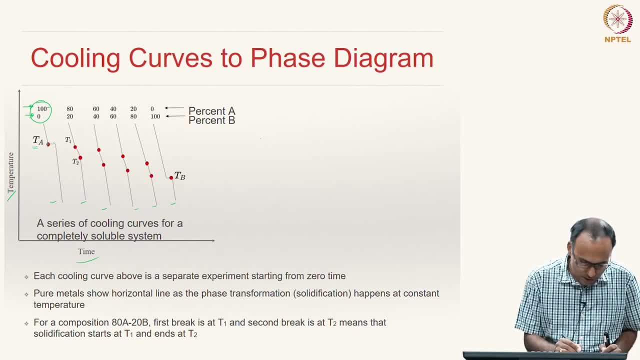 and it solidifies, And then so, during from here to here, it takes this much time for solidification, And then, completely after complete solidification happened, further cooling down takes place in the solid state. So here you have liquid, and here liquid to solid, and here you have solid right. 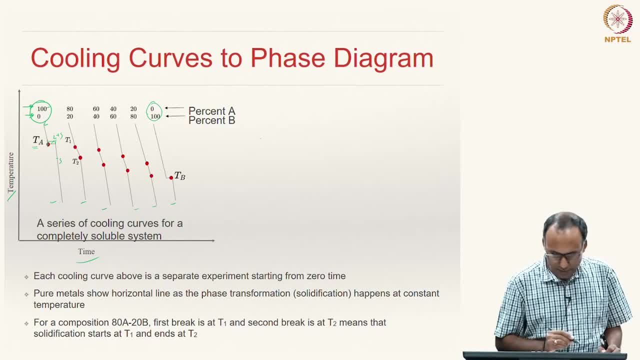 Similarly, the same thing happens for pure metal B. The pure metal B when it is cooled, when it reaches its melting temperature or solidification temperature T B, the solidification happens at constant temperature. So if this process is done then it increases the spent. 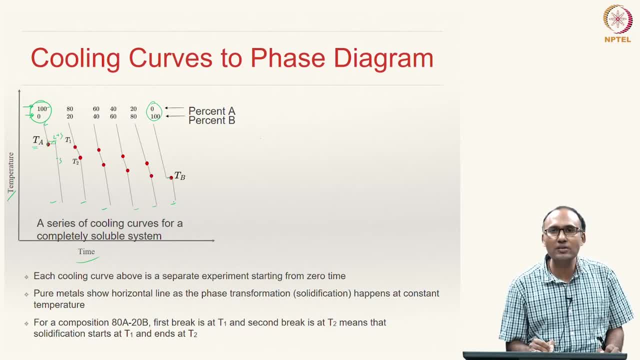 and then further cooling down happens in the solid state. Now, if you take any alloy in between, so 80,, 20,, 60,, 40,, 40,, 60,, 20,, 80, then what happens is the solidification, because 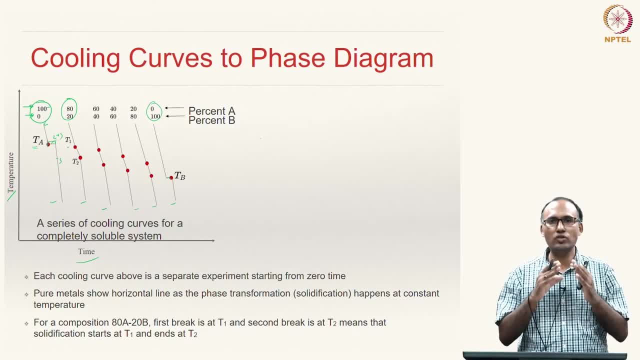 it is not a pure material. only for pure metals you will have solidification happening at constant temperature. The fact that it is not a pure metal: the solidification starts at a temperature, because here the solvent is A, and hence the solidification starts at a temperature just below T A, but close to T A, T 1- and then ends at a temperature T 2.. 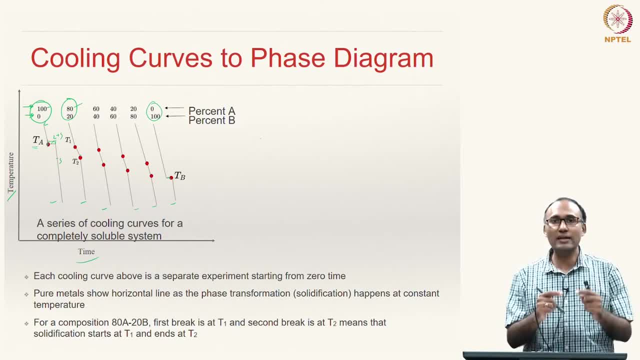 So that means here the solidification happens over a range of temperature rather than happening at constant temperature. The same, if you continue, if you see that for different alloys again, the solidification starts at a constant temperature, at a different temperature, ends at a different temperature, and so on as you move from this side to this side, the solidification temperature. 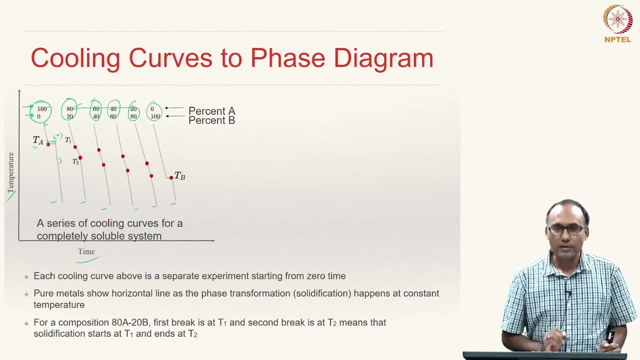 will be going on. So you are going closer to the solidification temperature of B when you are going from left to right, and now this is the point. So please note that for all these- although here we are showing time for all these- each of these curves, each of this cooling curve is an independent 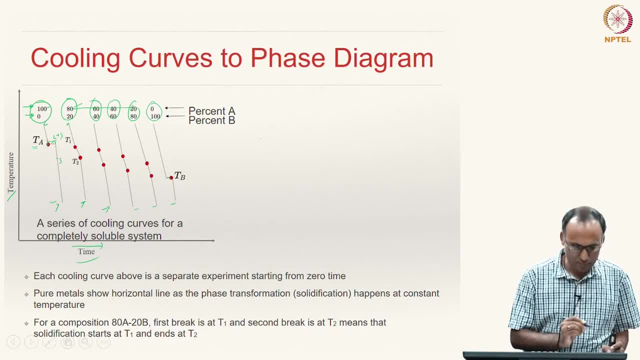 experiment. the time for each of them is 0 here. So just to show it on the same graph, we have shown the. shown it this way: Now, if you connect, So this is the composition, right. So now, if you would plot the same thing, if you know. 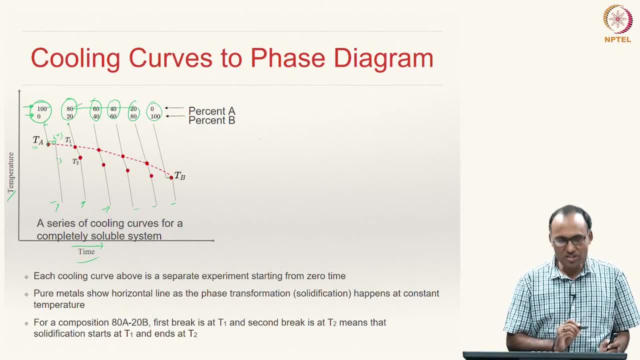 connect all the solidification start temperatures and the solidification end temperatures. the red dashed line represents the solidification starting and the blue represents the solidification ending. And we know that for pure material solidification starts and ends at same temperature, but for alloy any alloy in between. So if we have the solidification starts and ends, 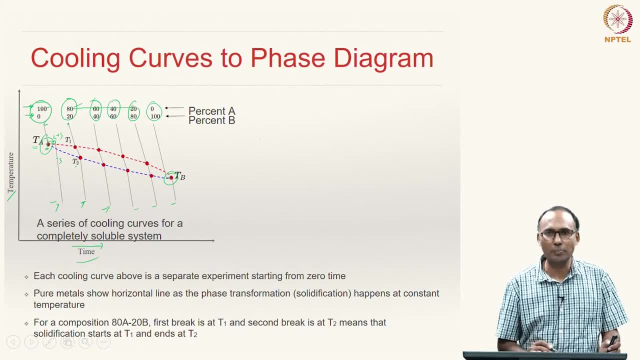 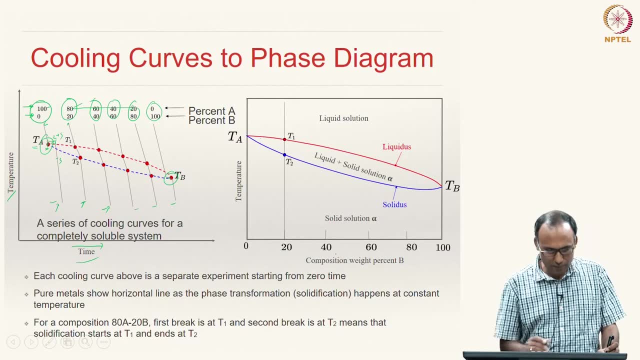 A and B, you will have a solidification happening over a range of temperatures. okay, Now, if you would plot the same thing on temperature composition diagram here we are showing, because its time it is slanted, but let us now assume that there is sufficiently long time that. 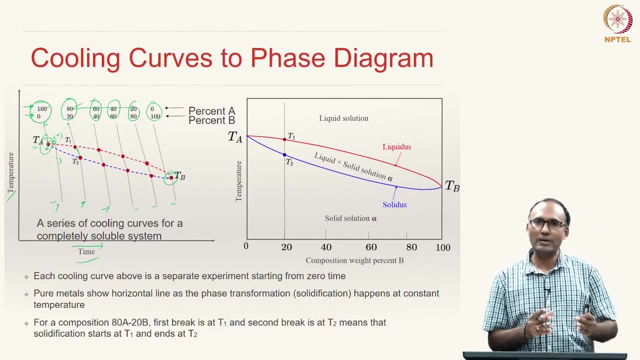 is given for this solidification to happen, So that the solidification is happening such that at each and every instant, equilibrium is maintained right. So now let us remove time from our picture and draw temperature versus composition, So at a given composition. 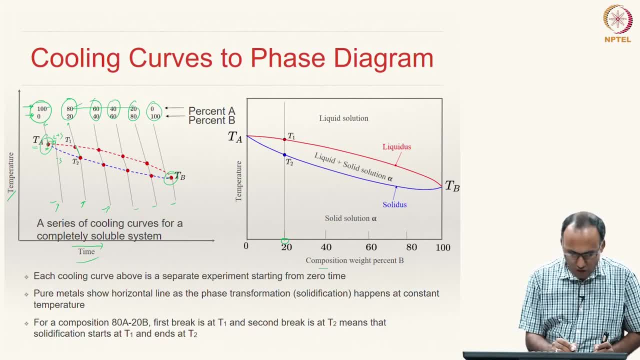 for 80, 20. that is this guy. the solidification happens over a range of temperature. The composition remains the same. that is why this is a vertical line. So this vertical line basically represents this process. Why is it vertical here? 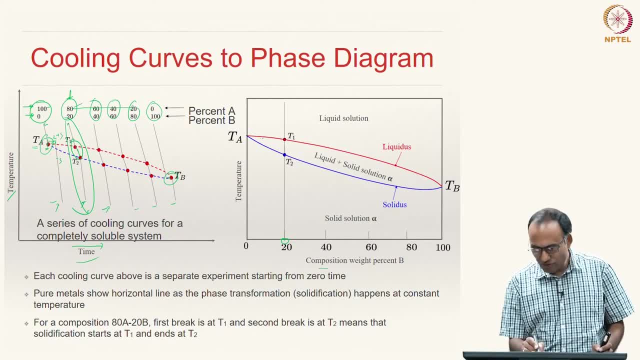 Because the composition of this direction is the same. So this vertical line is the composition is fixed Like that. if you draw for different ones, then you see that red curve is representing the boundary between liquid state to solid state. So because, above this, 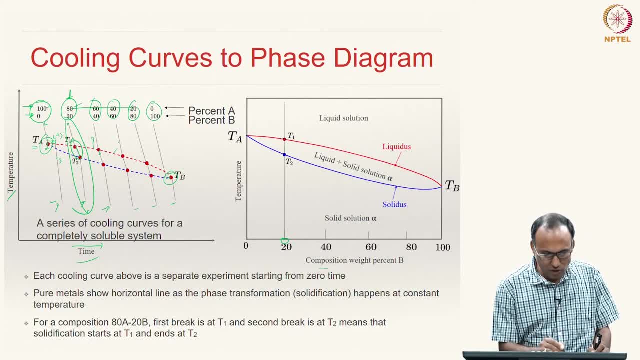 it is liquid, below this it is solid, right, So this is the solidification start temperature, solidification end temperature position. So this line, red line, is called liquidus. So this is the boundary between liquid state and solid state. So above this everything, 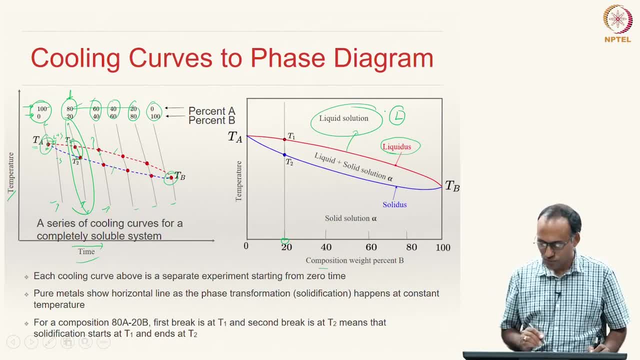 is a liquid solution, represented as L, and below this blue line everything is solid because the solidification is completed and below this is a. everything is solid, but it is not solid, it is a solid solution. So, in phase diagram terminology, all the solid solutions. 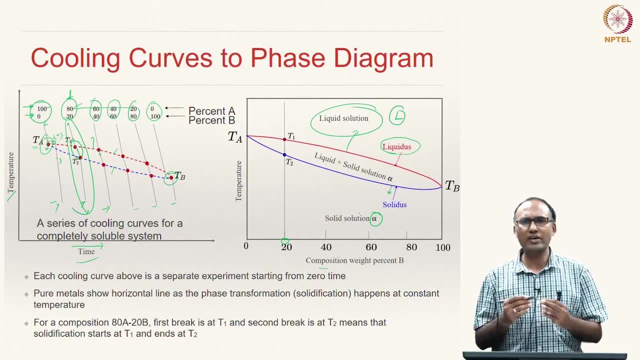 are represented by Greek letters: alpha, beta, gamma. whenever you see a Greek letter on a phase diagram, then it must be a solid solution. So in between, this line, red line is called liquidus line, this blue line is called solidus line. liquidus line is the boundary between liquid state and solid state and solidus line 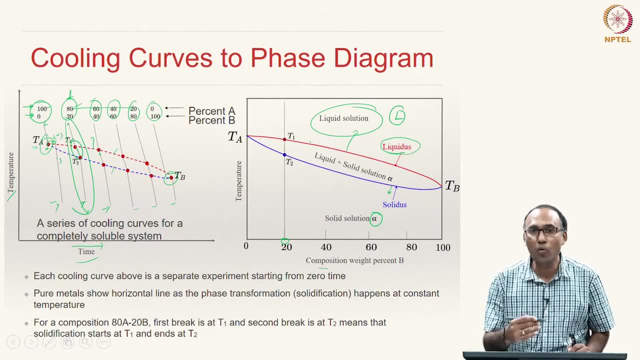 sorry. liquidus line is the line above which everything will be in liquid state. solidus line is the boundary below which everything, all the phases, will be in solid state. So here you have a, you have a liquid solution which is completely soluble. that means A is A and B are completely soluble in each other. So this is a single. 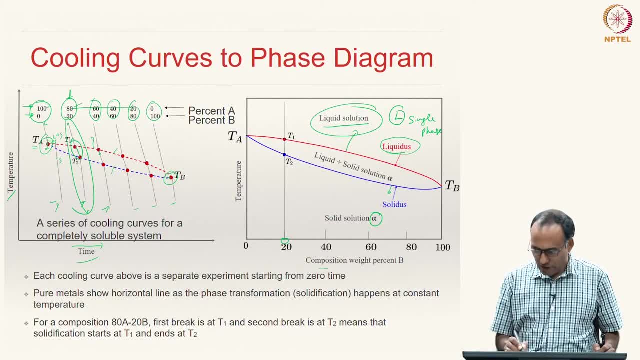 phase region. here you have a saying single solid solution phase. So this is also another single phase. here, of course, please note that the single phase region, but it may have two components. here also it is a single phase. alpha phase, that means a homogenous phase. with two components. So here you have a single solid solution phase. so this is also another single phase. So again this, I have Materiom here: qua Orion hike age H S is 0.5剛 mass alphaולם. Soşekkür ederim. 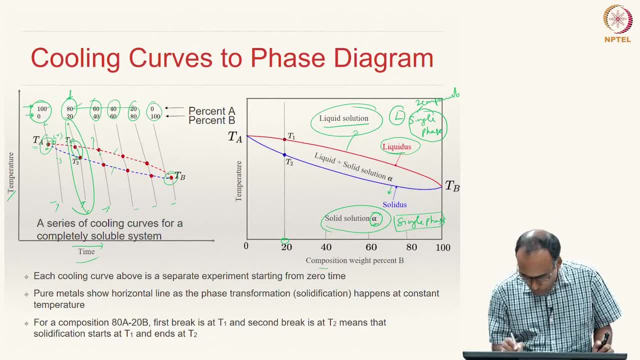 So the solid solution is of A and B. Now, if you, if you are looking at this region in between- and this region is a two phase region because there is some liquid and some solid solution, So liquid plus solid solution, So you have liquid plus solid solution. that 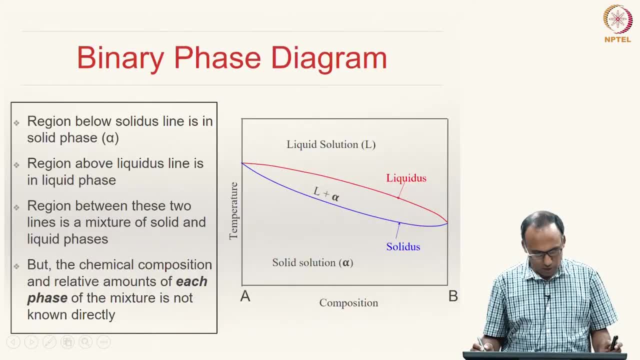 is what we call a two phase region. alright, So here I am summarizing. the region below the solidus line is called solid phase. The region above the liquidus line is called liquid solution, liquid phase. The region between these two lines is a two phase region. a liquid, 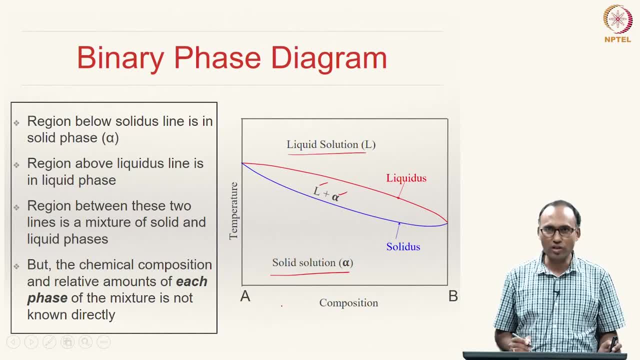 solution, a mixture of liquid solution and a solid phase, solid solution, alpha And know that we know in the liquid solution. suppose, if you are looking at a particular alloy composition, say let this particular alloy composition- So we know that liquid solution has a composition- say, let us say 20 B when we say composition of B, 20 B means A, T, A, because total together. 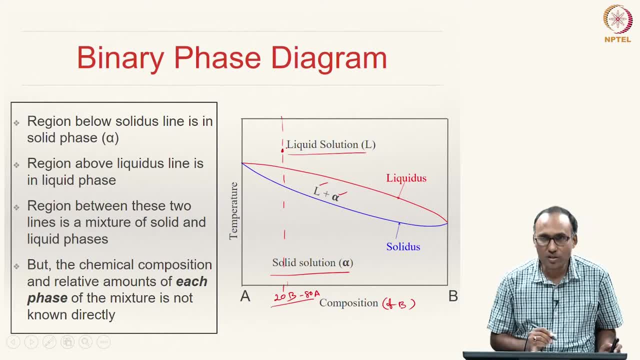 it should be 100, right, So 20 B. so that means this is the composition. here the composition is known because it is a single liquid solution. 20 B- Here also it is a single phase region, alpha- solid solution, alpha, which has a composition. 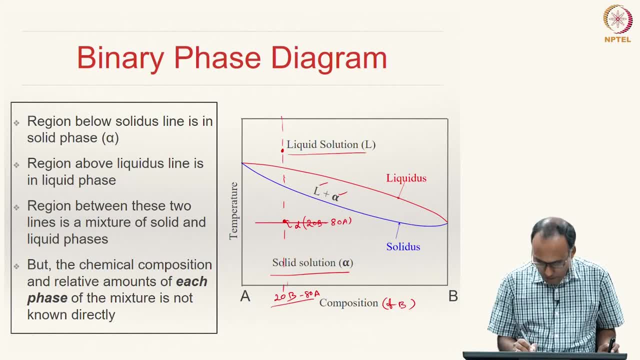 of 20 B, A, T, A, but now here it is a two phase region. We do not. now there are several thing that we do not know. what is that we do not know? you have a liquid solution, you have a solid solution: The composition of the liquid solution and the composition of the solid. 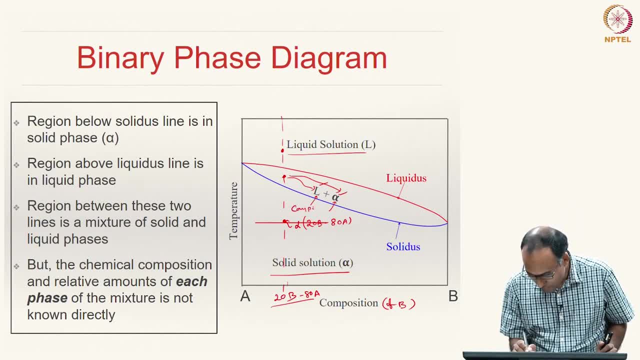 solution. compositions are not known. Will they be same or will they be different? That is something. The second thing is how much of the two-phase region mixture? what is the weight fraction of liquid phase and what is the weight fraction of solid phase? So their relative weight. 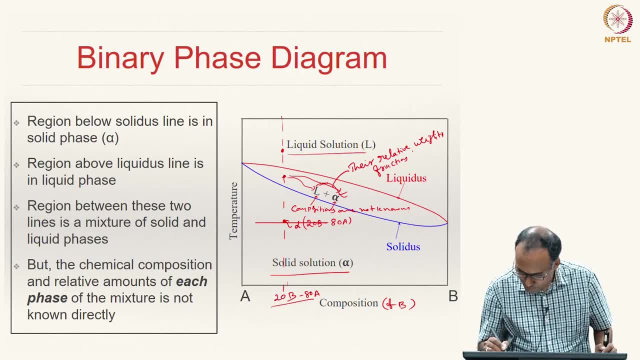 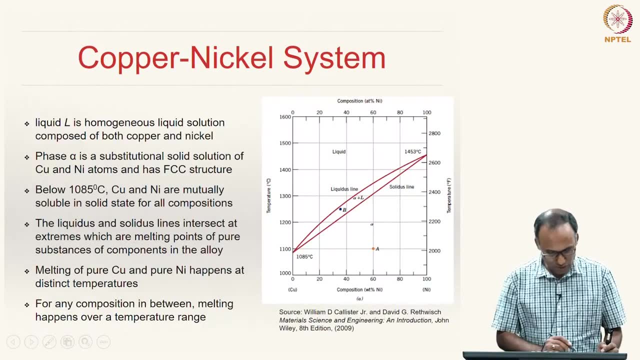 fractions or relative amounts are not known. That is what we are saying here, The chemical. so, in the region between the two-phase region mixture, what is the weight fraction of solid and liquid phase? It is the weight fraction of solid and liquid phase. That is the same. 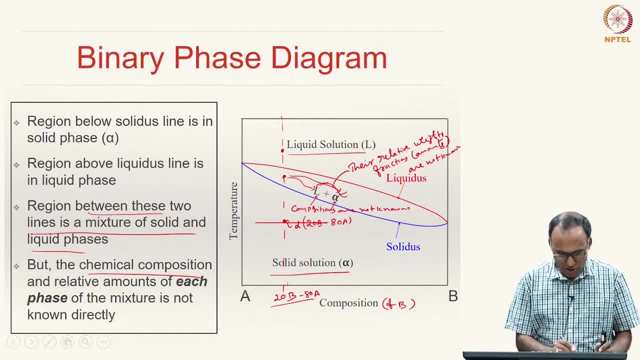 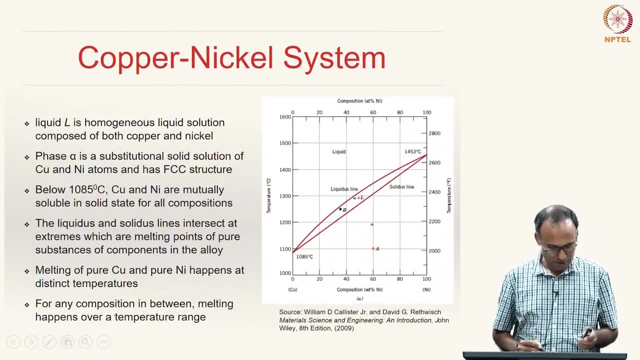 thing. We have seen this two lines is a mixture of solid and liquid phase, but the chemical composition and relative amounts of each phase of the mixture is not known directly. You need to do something about it. So here we are showing the phase diagram of a copper nickel system. Copper is a low 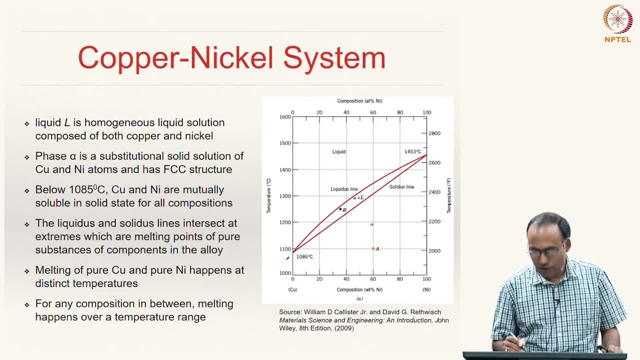 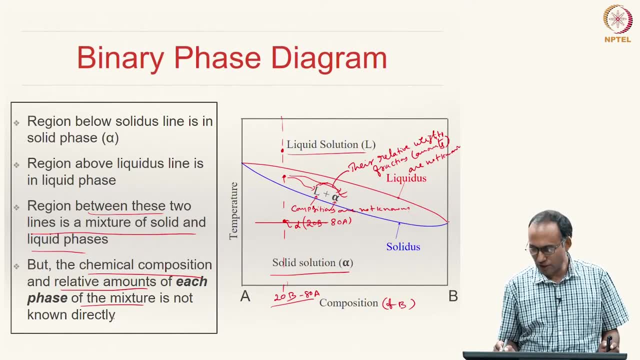 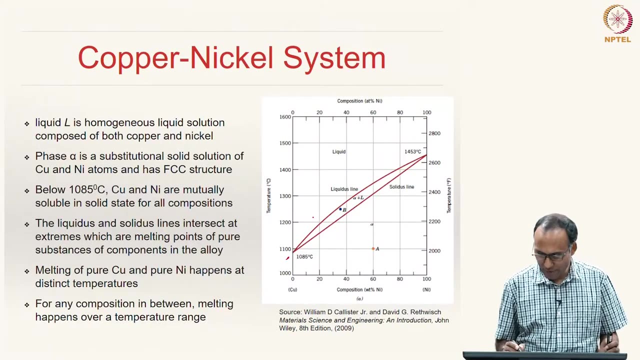 melting alloy, and nickel is a high melting alloy. That is why here previously, we have seen the phase diagram this way, but you can, instead of plotting the low melting point alloy on the right hand side, if you plot it on the left hand side. this is how it looks like This is a copper. 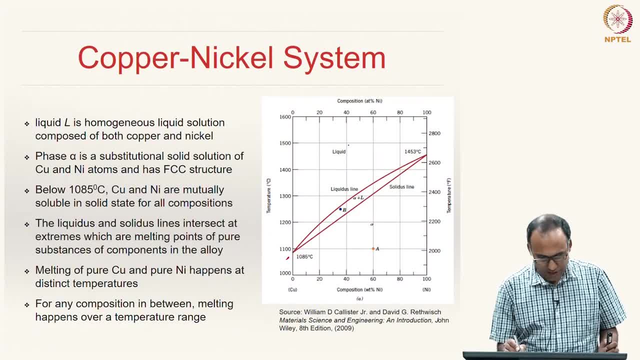 nickel alloy system and in this the liquid L region is a homogeneous liquid solution composed of both copper and nickel And alpha. so phase alpha is a substitutional solid solution, is a substitutional solid solution of copper and nickel atoms and it also has FCC structure. 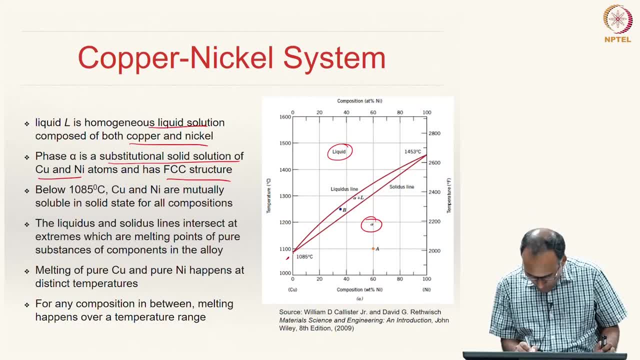 And now let us look at 1085 degree Celsius. Below 1085 degree Celsius, both copper and nickel are mutually soluble in solid state. for all compositions, For every composition, they are completely soluble in solid state And we can see that the melting point alloy 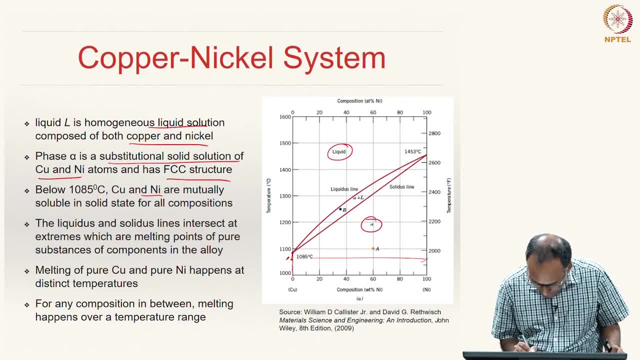 of copper is 0, 1, 0, 0, 0, 0, 1, 0, 0, 0, 0, 0, 0, 0, 1, 0, 0, 0, 0, 0, 0, 0. 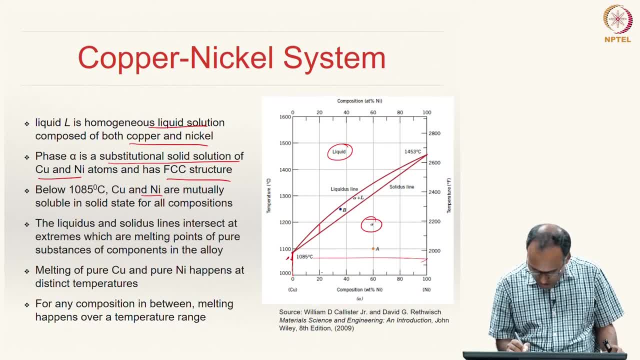 So those are the two components that are being discussed. So for the melting of copper, for the melting of pure copper, suppose, if you take solid copper and if you are heating it up the melting happens at constant temperature. and also for pure nickel. But for any alloy the melting happens over a range of temperatures. For for instance, this particular alloy, which is 20 nickel, happens over a range of temperature- let us say this is 1150 and this is about 1190- over a range of temperatures 1150-1190, the melting happens. 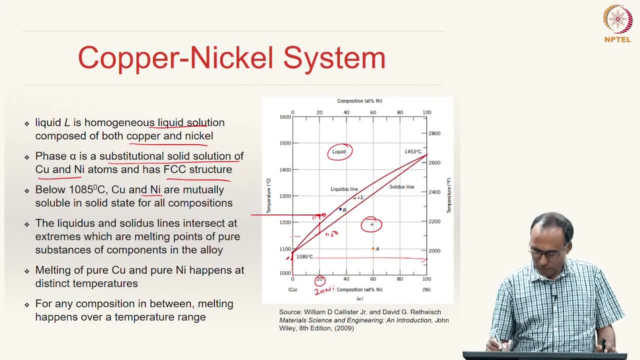 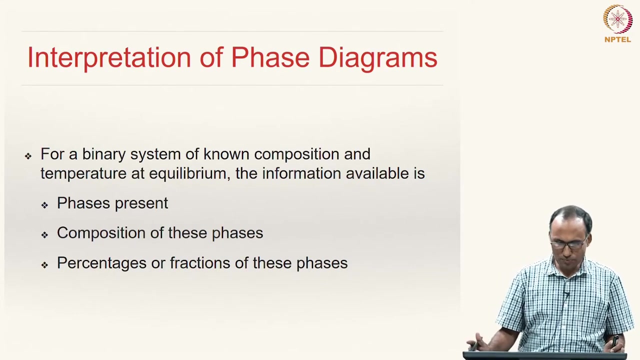 So the liquidus line and solidus line, this is our liquidus and this is our solidus line. they intersect at extremes, which are the melting points of your components or pure substances. So how do we go about interpreting the phase diagrams? So by a binary system? 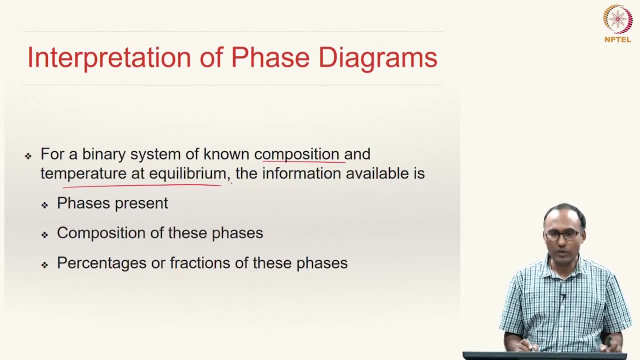 of known composition and temperature at equilibrium. we have the following information: What is the information that we have For a given composition and a temperature? we know what are the phases present, whether it is a single phase region. if it is a single. 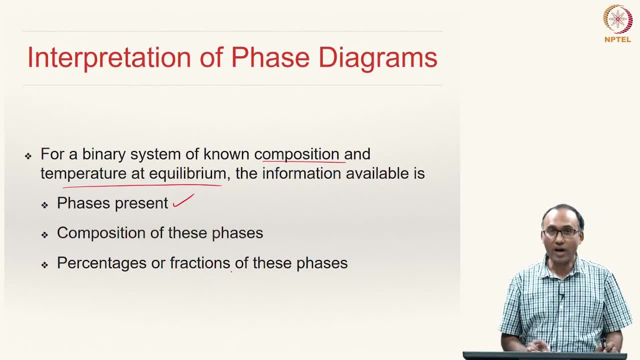 phase region, whether it is liquid phase or a solid phase, or is it a two phase region, And we need to understand if it is a two phase. if it is a single phase region, the composition of the phases is known And but if it is a two phase region, of course we need to find out what are the compositions. 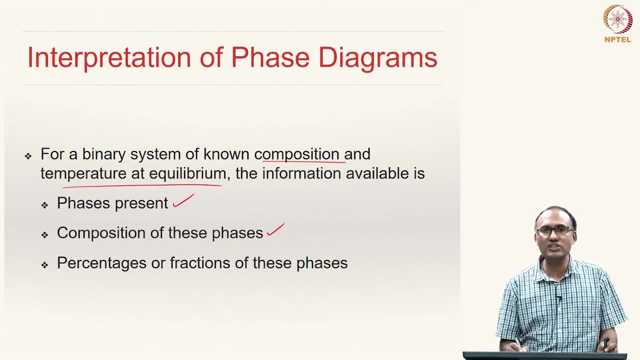 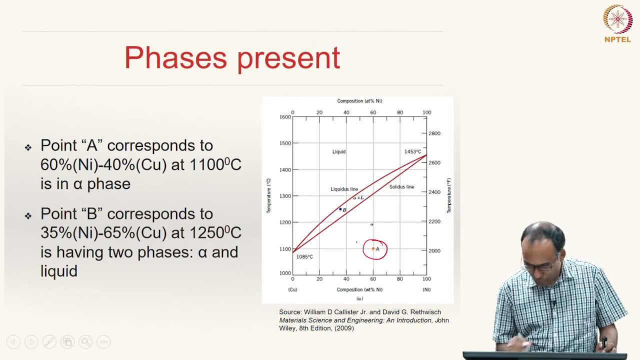 of these individual phases and what are the percentage or fractions of these or amounts of the individual phases. So, for instance, in this phase diagram you see the point A. Point A corresponds to 60 percent nickel, 40 percent copper at 1100 degree Celsius and 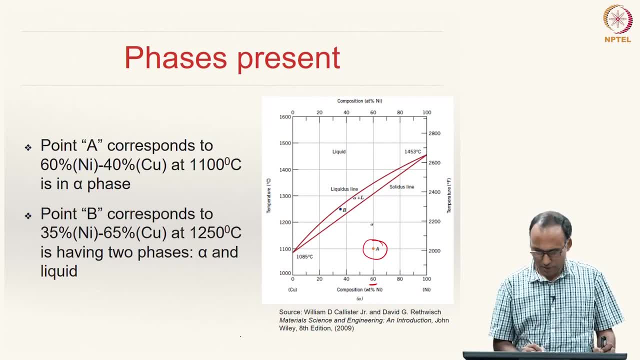 which is in alpha phase. it is a single phase region. However, point B here, which is a two phase region, corresponds to about: this is 30, so it is about 35 percent nickel, 65 percent copper at 1250 degree Celsius, but having two phases, that is, alpha and liquid. 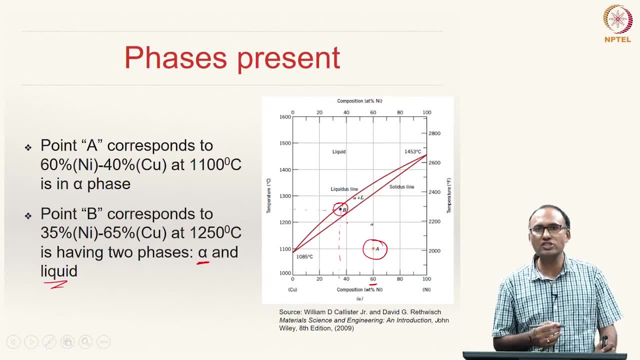 solution, So liquid, also a liquid solution. it is not pure A or pure copper or pure nickel. it is a solution of copper and nickel. So you have alpha phase and liquid phase. There are two phases that are present at B. 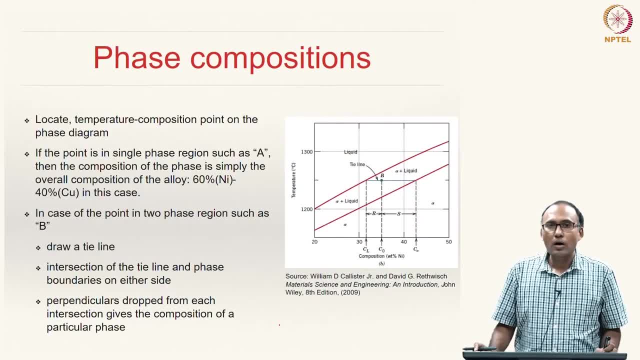 All right, And now, what are the compositions of these phases? So in the two phase region at B you have alpha and liquid. What is the composition? So the way that one needs to find out the composition is at this: 1250 degree Celsius, you draw a horizontal line that represents 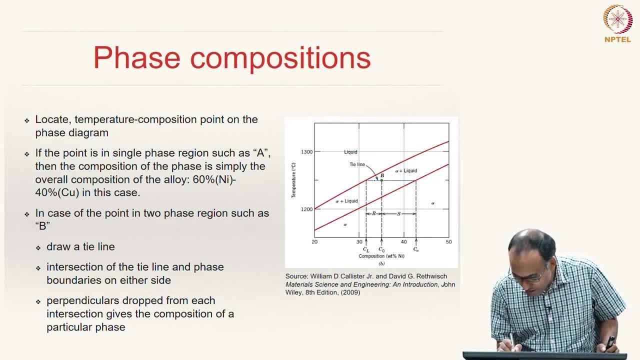 the constant temperature line and wherever this, this line, is called tie line, the horizontal line that is drawn in the two phase region is the tie line. And wherever this tie line hits the liquidus, this is our liquidus right and that is our 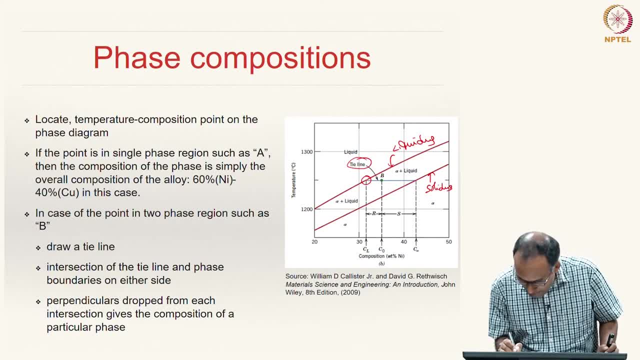 solidus, Wherever that hits the liquidus, and you draw a, drop a vertical and that represents composition of the liquid phase that is present. wherever this tie line hits the solidus, drop a vertical. that represents the solid phase of the C alpha here, composition of the solid phase present. That is how we can find out. 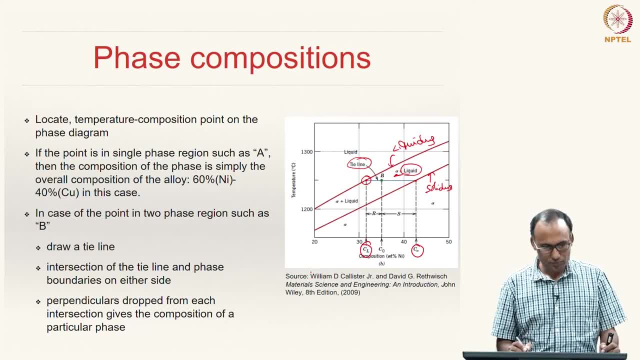 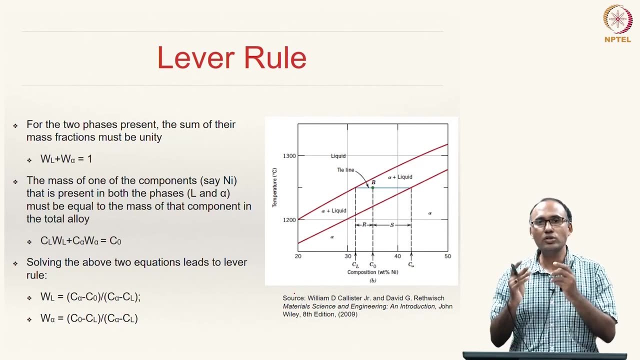 the compositions of the phases, as that is what we have clearly written here, So you can go through the text later. And now, how about…. So we know the compositions, but how do we find out the amounts? What is the quantity of liquid that is present? What is the quantity of solid fraction of the liquid? 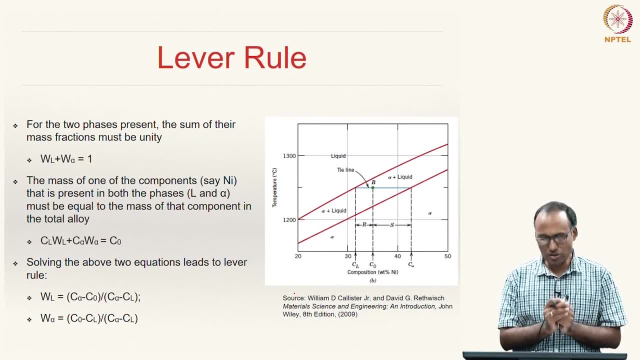 that is present, What is the fraction of the solid that is present? For that we use something called lever rule. So what is that lever rule? So for the two phases present, the liquid and alpha sum of their mass fractions, or weight fraction, should be equal to 1.. So 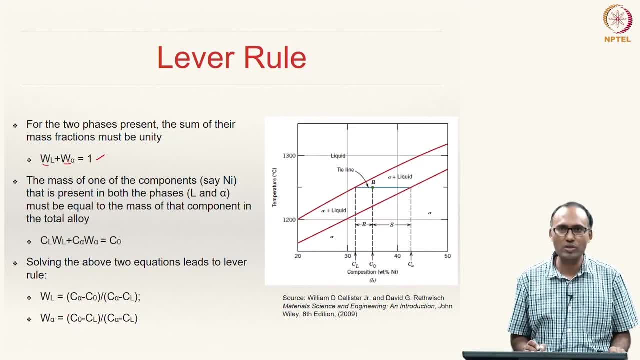 weight fraction of liquid plus weight fraction of alpha solid solution must be equal to 1, right Now, the mass of the one of the components, say nickel… So one of the… So in both phases you have both the components, The components. 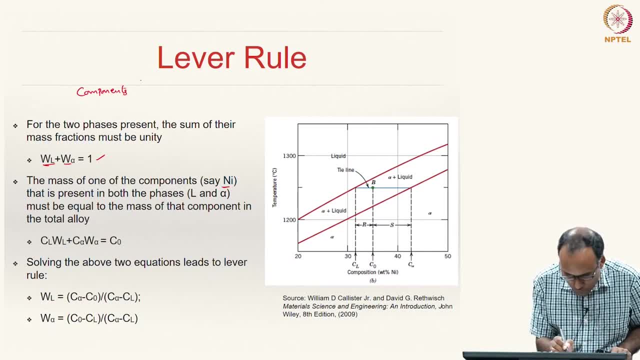 are what Copper and nickel. This copper and nickel is present in both liquid and alpha phase. In liquid also. you have copper and nickel. Alpha also, you have copper and nickel, right. But now let us say that the mass, fraction of mass, of one of the components say nickel. 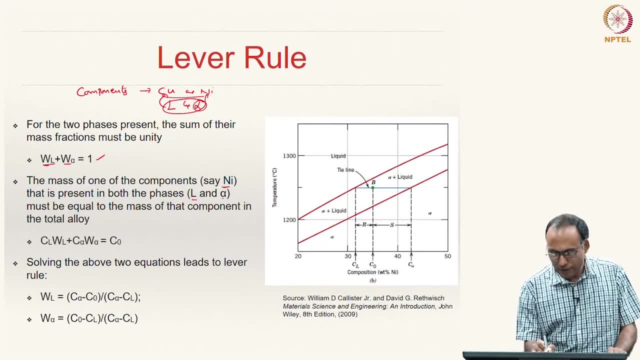 is present in both the phases, present in both the phases, That is, liquid and alpha. So you have: in liquid phase there is some nickel, In alpha phase there is some nickel right. So now we are saying that the mass fraction or the mass of the component B or 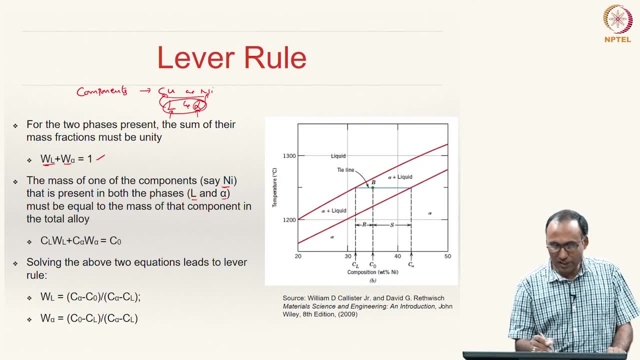 component A, For instance, in this case nickel, present in both the phases, must be equal to the mass of that component in the alloy, is not it? So you have this alloy In this alloy, the mass of the… the alloy, The mass of the alloy, is present in both the phases. The 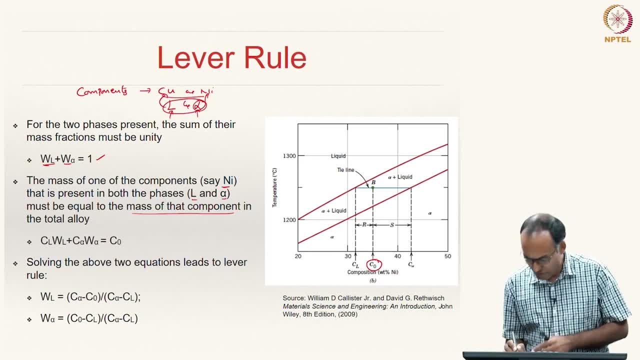 nickel is C naught. right, that is the weight fraction. So C naught is the mass of the liquid. Then the nickel should have been: this is the amount of nickel that is present in this alloy and that should have been distributed into alpha and liquid. So then it means the 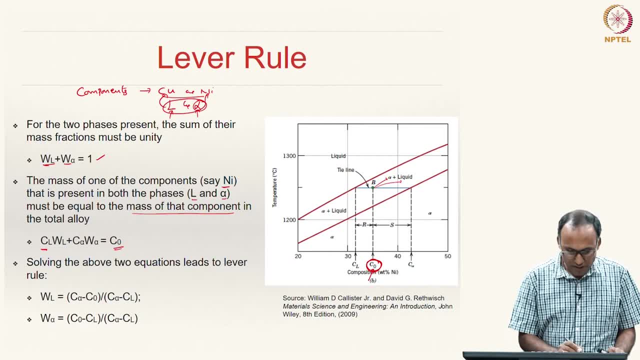 composition in the liquid phase. composition of nickel in liquid phase times: weight fraction of liquid plus. composition of nickel in solid phase times: weight fraction of solid to be should be equal to the weight fraction of the nickel alloy that we are looking at, this particular alloy, That is, the total weight fraction of the nickel in that alloy. Now, 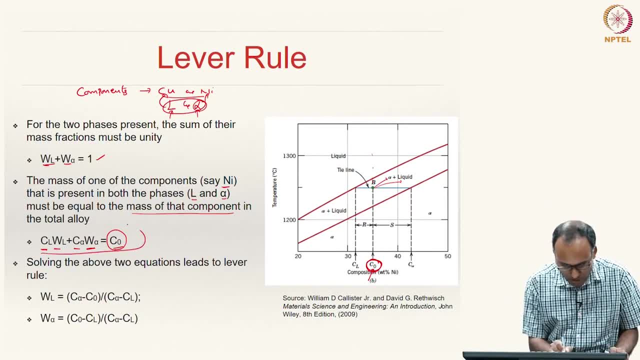 that is distributed into liquid phase and solid phase. So this should be true. Now, using these two equations, we can find out what is the weight fraction of liquid, what is the weight fraction of solid. So that is C alpha minus C naught by C alpha. 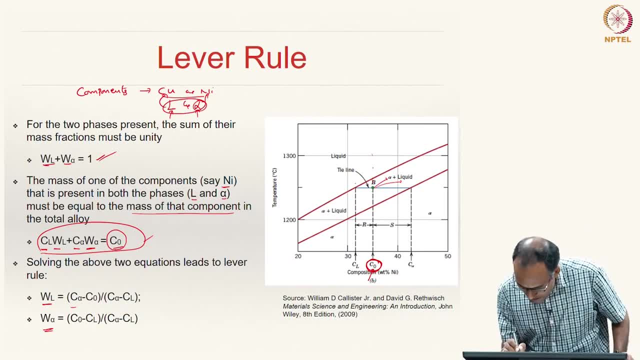 minus C L. So what is C alpha minus C L? C alpha minus C L is the total length of this tie line. right, That is our C alpha minus C L. That is the length of the tie line. Now we want to find out what is the weight fraction of the liquid. We know what is the composition. 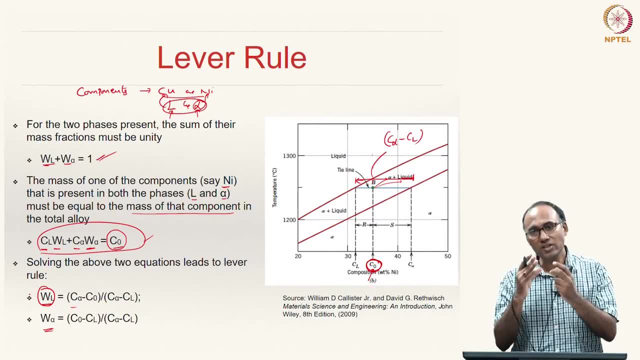 of liquid phase and solid phase. Now, what is the weight fraction of the liquid out of this total? How much amount of liquid is there? That is C alpha minus C naught. What is C alpha minus C naught? That is this. 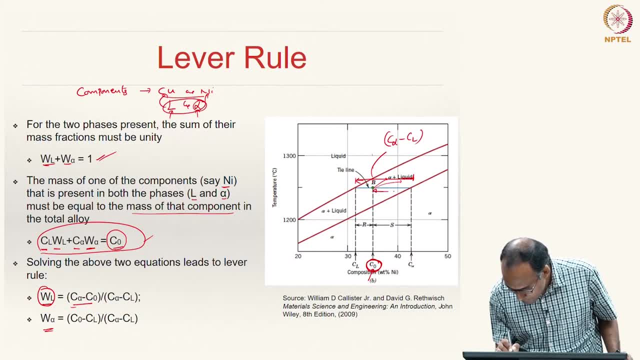 distance. This is C alpha minus C G L divided by the total distance. Take c alpha minus C L, mouth toute distance of C Apple minus C L And I will write n plus c alpha minus c 0 as c 1. And you will have to keep this substitute one. So if you want a constant, 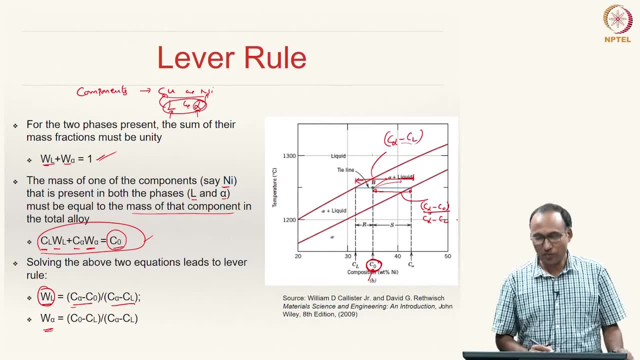 at the end of this entire viene, you have to write c alpha minus c 0.. That means if you want, means if you want to find out the weight fraction of the liquid. So now you are. at this point, you have drawn the tie line. all that you need to do is this is the liquid. 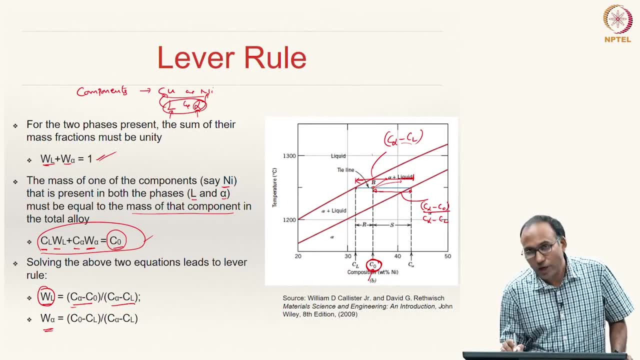 s line, right, So liquid is on this side. So what you have to do is you have to take the length of this tie line from the point B to the solid s line, So this other side line divided by the total length. similarly, if you want to find out the weight fraction, 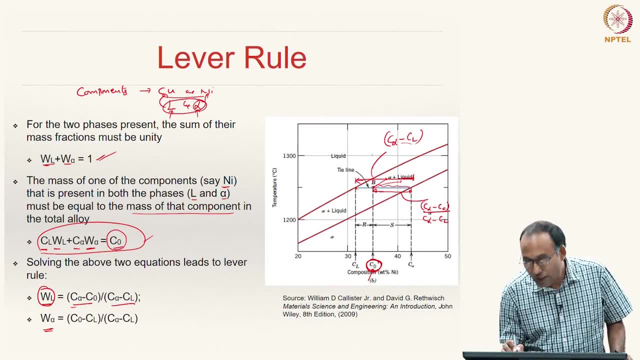 of the solid. weight fraction of the solid will be the length of the tie line, from the point, the, where we are looking at the composition, to the liquid s line. So that is this length divided by the total length, right? So that will give us weight fraction of the solid. 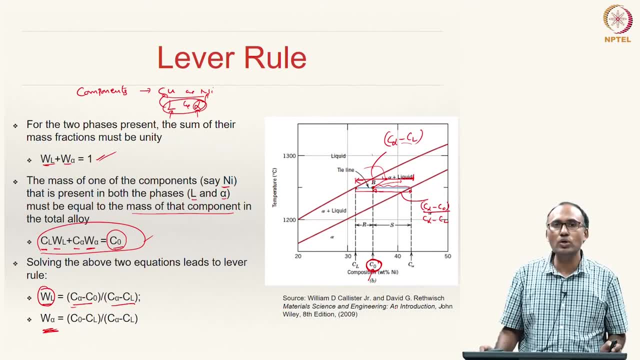 So, in this, this is the thing that one needs to do in the two phase region, because there are two phases present, and hence we need to know what is the weight fraction of solid and what is the weight fraction of liquid, Whereas in the single phase, 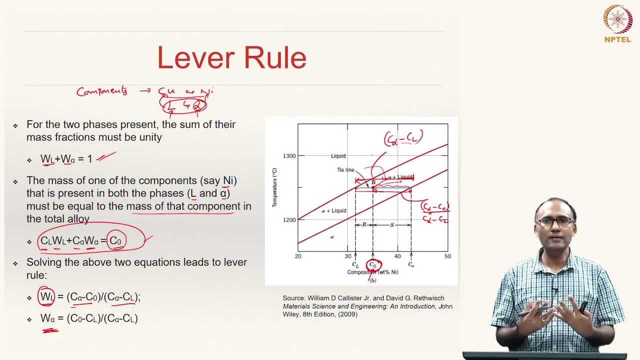 Single phase region, 100 percent will be that particular phase right. There is no reason for us to use the tie line or lever rule, because there are no. there is only one phase that is present and hence all the weight fraction will be of that one and the alloy composition. 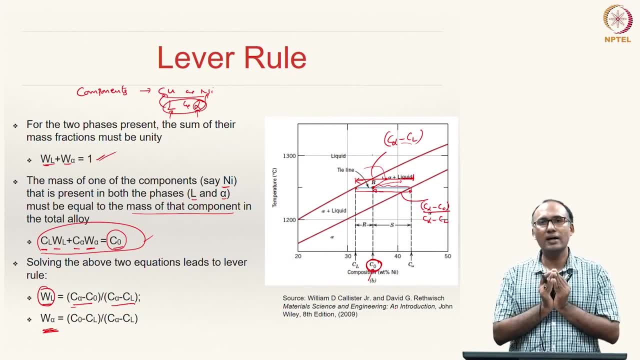 will be the composition of the as a single phase region. The reason why we need to do that in a two phase region is because there are two different phases and each phase how much weight fraction is present, and each phase- This is what is the composition is something that one needs to find out, alright, So for 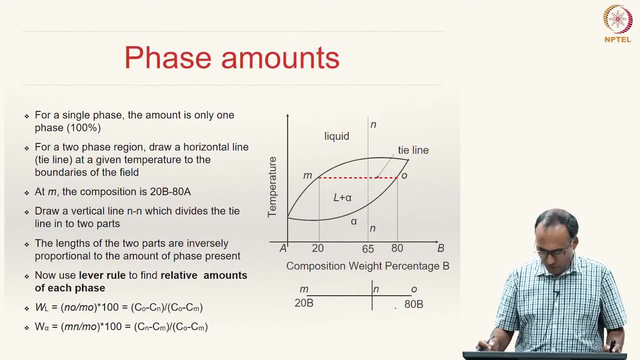 example, in this, if we are looking at a 65 percent B situation, right, all that you need to draw, you have to take You- let us say you are interested in this point- all that you need to draw is a: draw a horizontal line m n. So today you now interested in, as you. 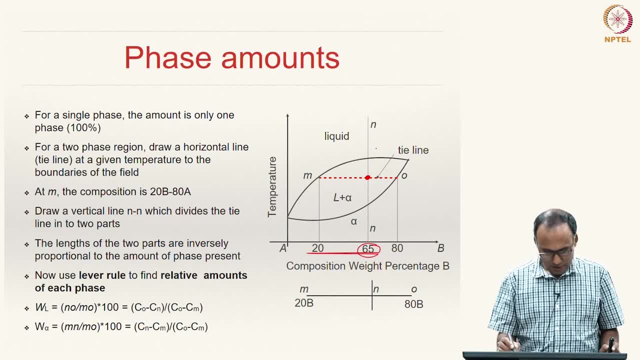 read the line, Writing a horizontal line such that I get two orders in this line, But if m, n, m, o and then the distance, Now all that we need to do is, in order to find this, will be: this is our liquidus line, this is our solidus line. So the composition of liquid. 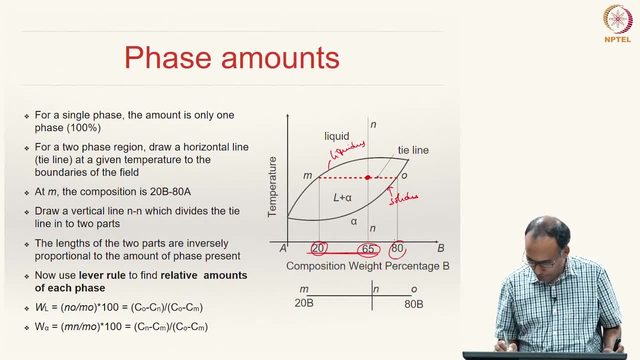 will be 20 b. composition of solid will be 80 b. the weight fraction of liquid- let us say this point- is p, the weight fraction of. So let me say this point as n, not p? n the weight fraction of liquid will be: this is liquidus line and hence you need to take the. 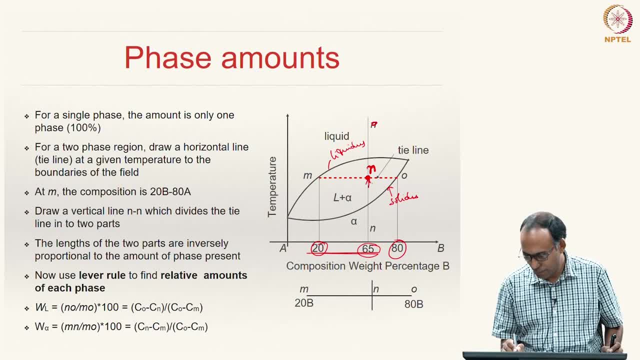 other point. This is called lever because it is like fulcrum, about which it is oscillating. So this is n? o divided by m? o should be giving us the weight fraction of the liquid. So n? o divided by m? o. 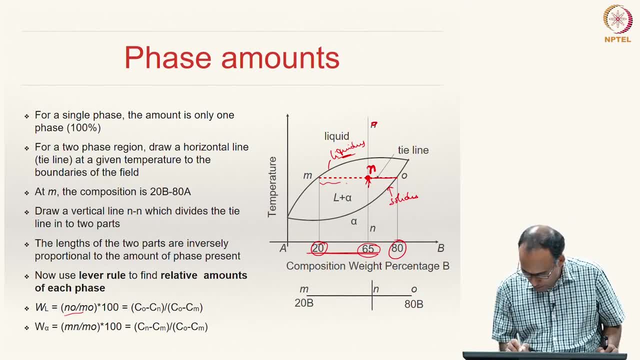 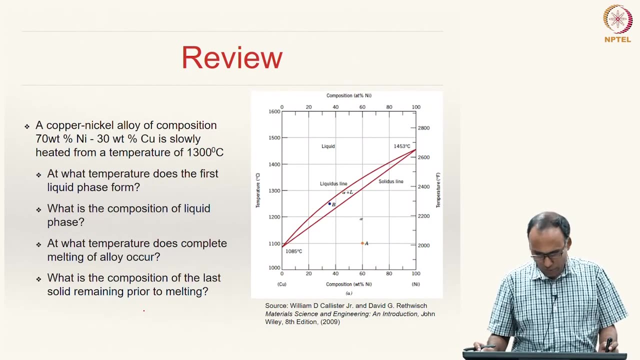 Similarly, the weight fraction of solid should be. this is the solidus, So, and hence you have to take the other side. So m? n divided by m? o, that will give us the weight fraction of the solid. So let us review once again. You have a copper nickel alloy of composition. 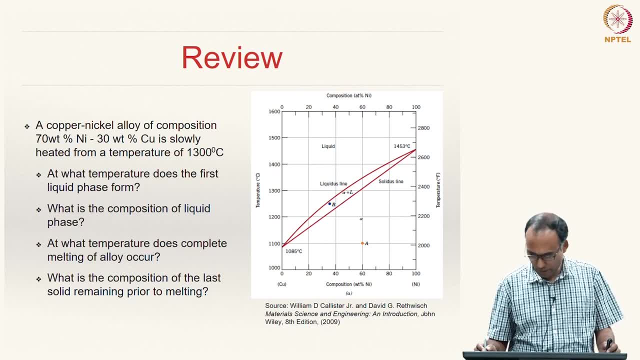 70 weight percent nickel and 30 weight percent copper. Where is 70 weight percent nickel? That is this guy, So we have. This is the alloy that we are looking at. It is slowly heated from a temperature of 1300 degree Celsius, So here, initially, it is at this temperature, From that temperature. 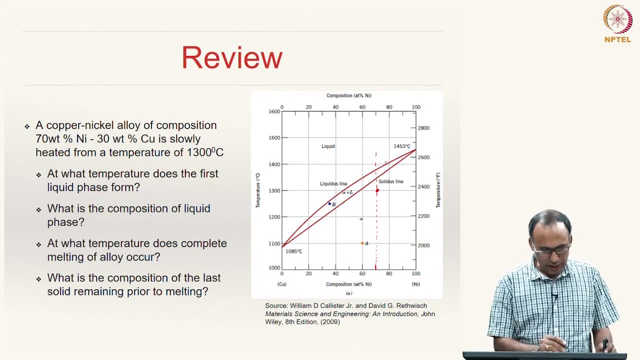 it is slowly heated And the question is: at what temperature does the first liquid phase form? So when you are here it is a solid state, and when you are entering here at this temperature the first liquid phase starts forming right. So that is about� So 13,. 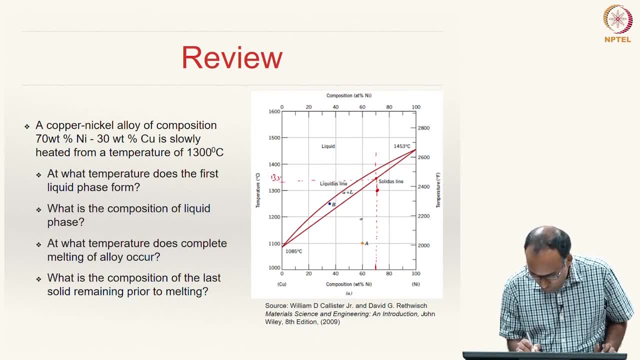 here, it is approximately right. So that is the temperature at which the liquid phase starts forming. What is the composition of liquid phase? So if you are in this regions, so if you draw a small tie line there, so that will be the composition of this겠죠. So if you draw a small tie line there, so that will be the composition of this. So for the in this form, and that explains this first liquid phase ends. But in thisften let me just stay few minutes. Let me write down some of these, mainly because they are less important. All right, So if we are in this region, and we are in this region And you write down theặt, we are deciding which liquid. the small liquid phase that is forming initially- So that will be about this- is 50 and this is 58 percent nickel. At what temperature does complete melting of alloy occur? If you go upper, if you continue to heat it up and let us say this is 1380.. At 1380 degree Celsius. 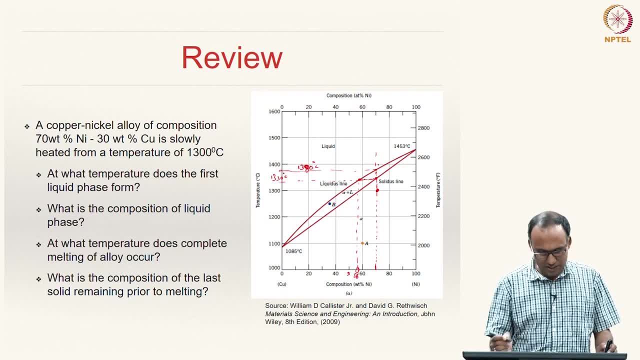 the complete melting of alloy occur and then it will be in complete liquid state. What is the composition of the last solid remaining? Just below this line will be the last solid remaining, So you have to, in the two phase region, draw a tie line. So that will be the. 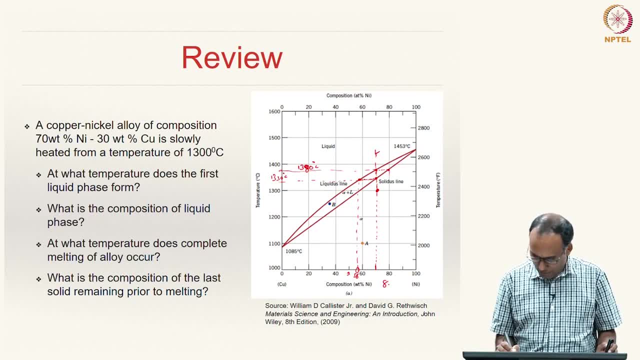 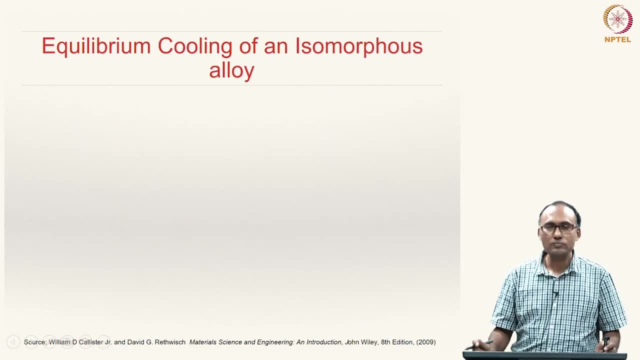 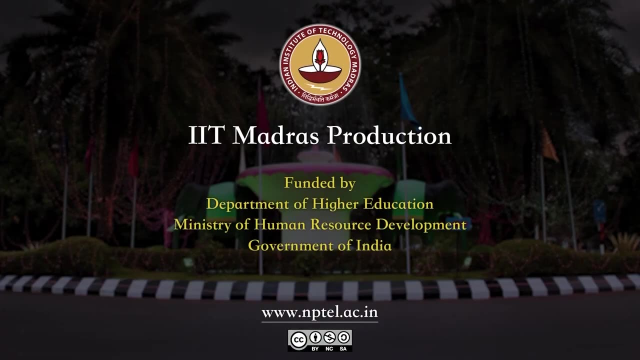 composition of the last solid remaining, and that will be 80 percent nickel. With that you can work out the composition of the last solid remaining. So this is the composition of the last solid remaining. So find out all the weight fractions and then compositions of an alloy.